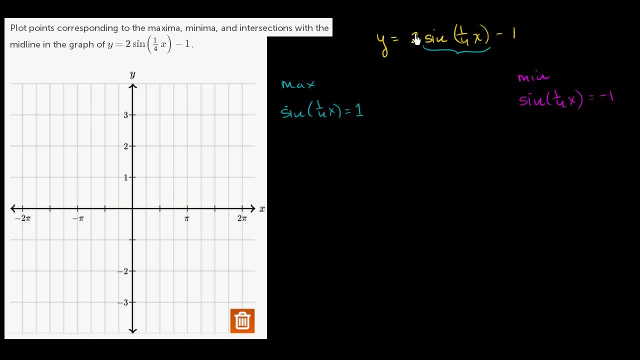 hits the point, negative 1.. And, of course, when it hits this point, we're then going to multiply: it times this 2.. So the maximum value of this part of the expression is going to be 2 times 1, the maximum value of the whole function. 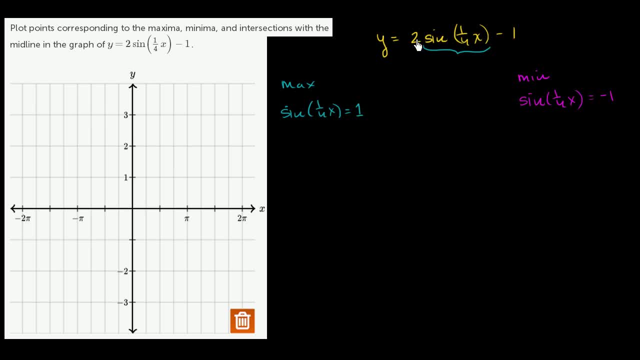 It's going to be 2 times 1 minus 1.. The minimum value is going to be 2 times negative: 1 minus 1.. But we'll get to that. Now, what about when we intersect the midline? We intersect the midline whenever this part of the function. 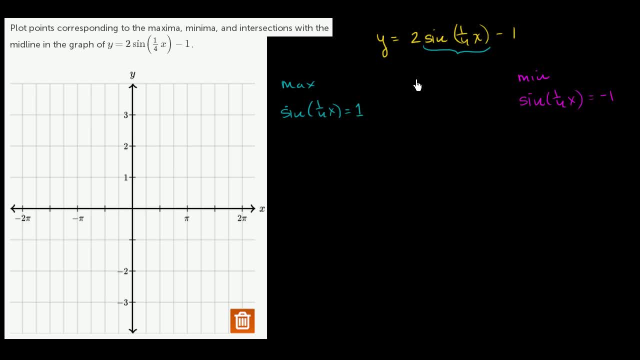 is equal to 0. And we're essentially just left with that part right over there. So let me write this Midline: and this is going to be 0 when sine of 1, fourth x is equal to 0. So when do these things happen? 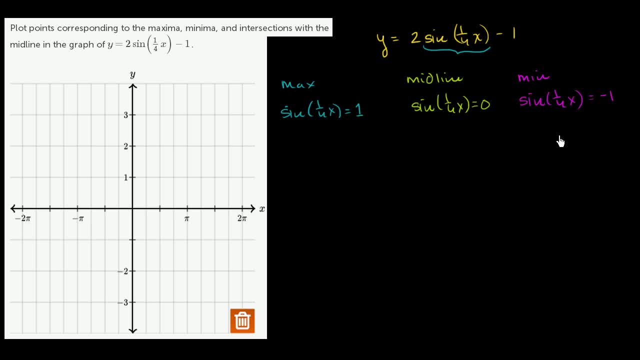 When does the sine function hit 1?? When does the sine function hit 0?? When does the sine function hit negative 1?? And to think about that, I will draw ourselves a little unit circle to help us visualize things. So a little unit circle. 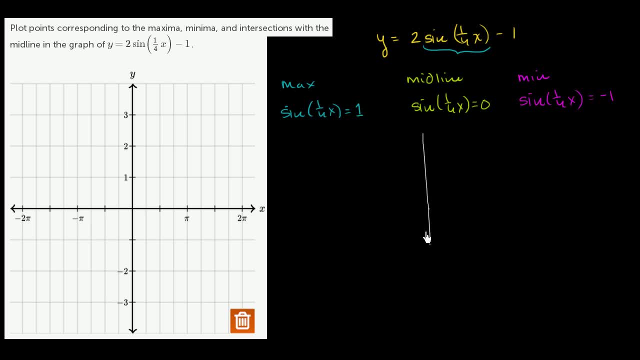 I don't want to make it too little so that we can. So a little unit circle right over there- That's our y-axis, That is our x-axis, And it's a unit circle centered at the origin- has radius 1.. 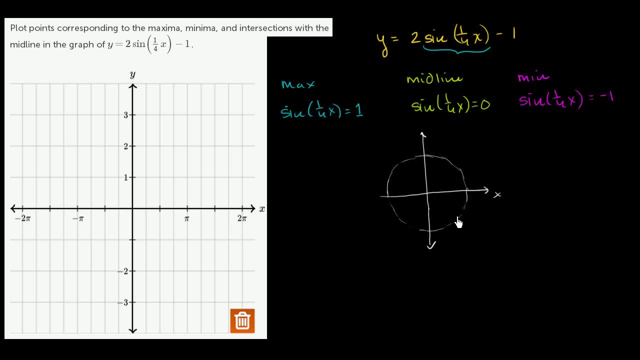 So, just like that, Just like this, And this, of course, is the point negative 1.. Sorry, this is the point 0, negative 1.. This is the point 1 comma 0.. This is the point 0 comma 1.. 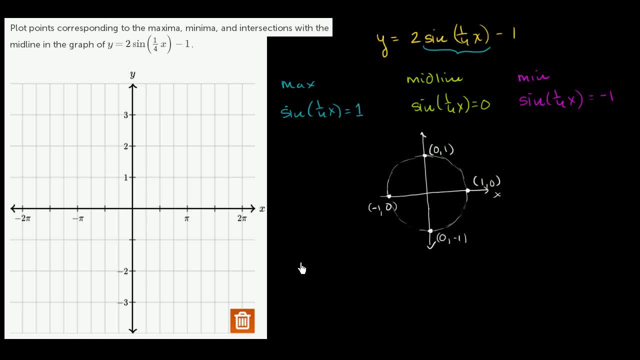 This is the point negative, 1 comma 0.. Now let's start with an angle of 0 radians, So we're going to intersect the unit circle right at that point, at the point 1 comma 0. And remember the sine evaluated there. 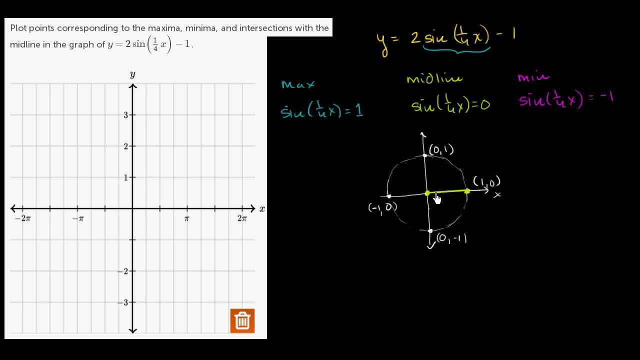 by the unit circle definition of trig functions is going to be the y-value. So we see sine of 0 radians is equal to 0. And not just 0 radians, any integer multiple of 2 pi plus 0 radians. So we could add 2 pi. we'd go around again. 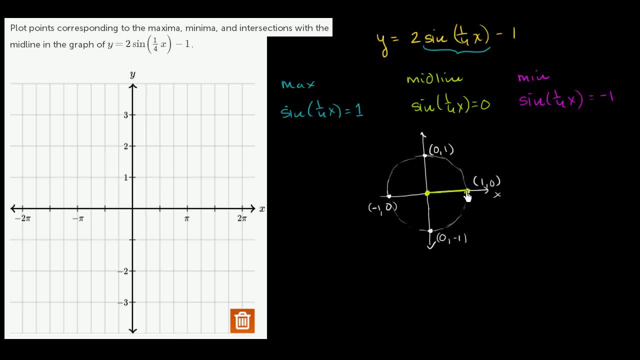 we'd get to the same point: add 2 pi again. Now we've added 4 pi, we go again. We could subtract 2 pi And we're back there again. So this is going to happen whenever, whatever we input into the sine function. 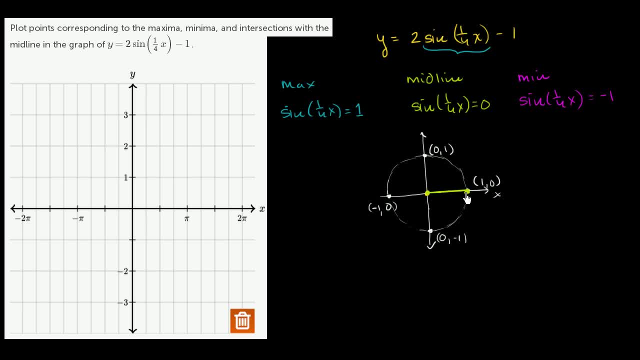 is equal to 0 radians plus some multiple of 2 pi radians. So when is this going to be equal to 0?? Well, when 1 fourth x meets that constraint. So that's going to happen whenever 1 fourth x is equal to 0, plus or minus. I guess I could say: 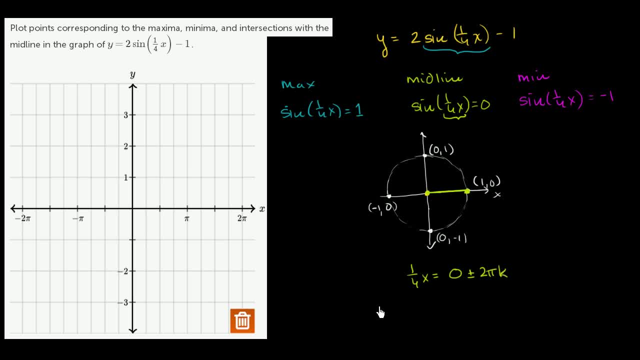 2 pi times or some multiple. And remember all I'm saying here is if you input anything like this into the sine function, you're going to be at this point on the unit circle And when you evaluate the sine of the function, 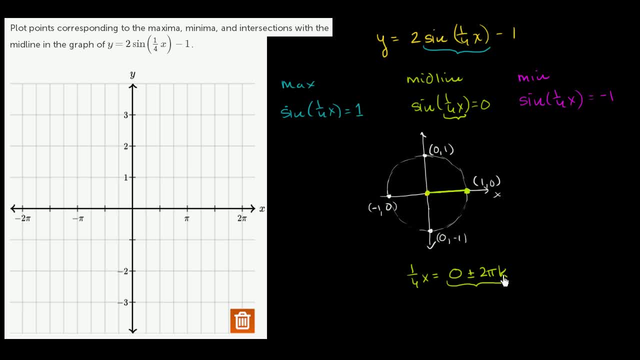 at any of those points you are going to get 0.. Why did I write k here? Well, this is just for some integer k. So this is just saying 0 plus 2 pi, 0 plus 4 pi, 0 plus 6 pi. 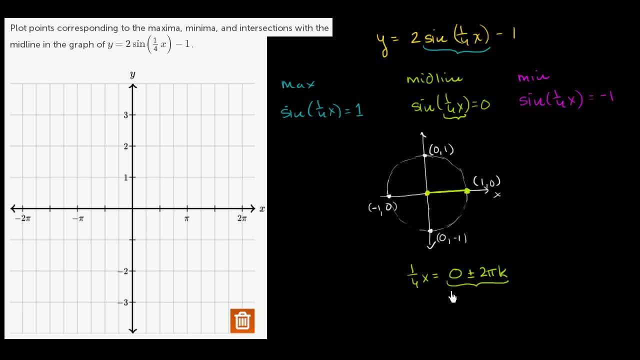 0 minus 2 pi. This encapsulates all of that. So let's solve for x. Well, to solve for x, we just multiply both sides by 4. We get: x is equal to 4 times. 0 is 0 plus or minus 4 times. 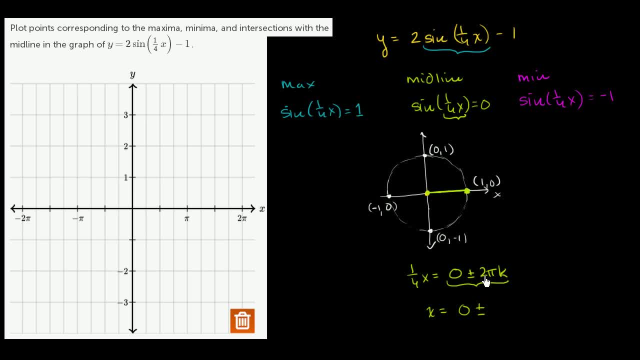 some multiple of 2 pi would get us, or 4 times 2 pi k is going to give us 8 pi k. So now it's going to be, when x is 0 plus or minus any integer multiple of 8 pi, this whole function. 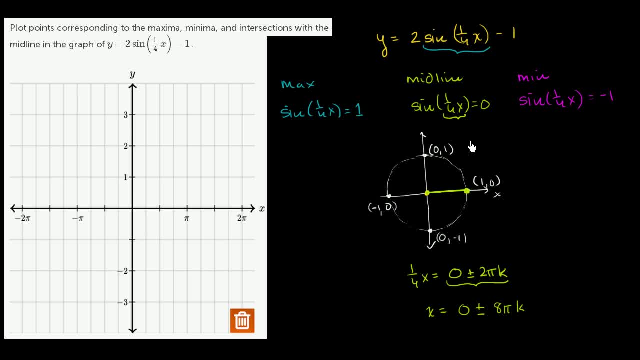 is going to intersect the midline. Why? Because when x is any of these things, when you input any of these x values there, you multiply it by 1. fourth, you evaluate sine there. then this whole expression is going to be 0. 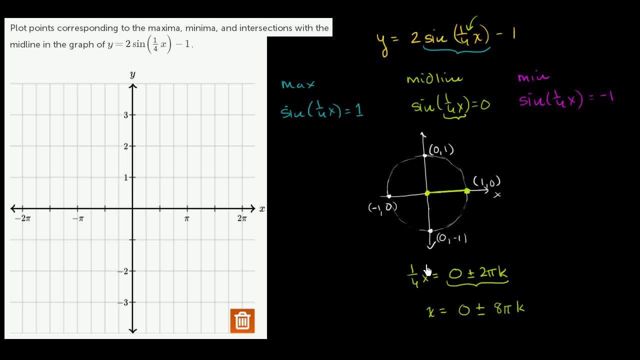 We're going to hit the midline. y equals negative 1.. So let's just go with the simplest one. Let's just go with x equals 0. When x equals 0, all of this stuff is 0.. y is equal to negative 1.. 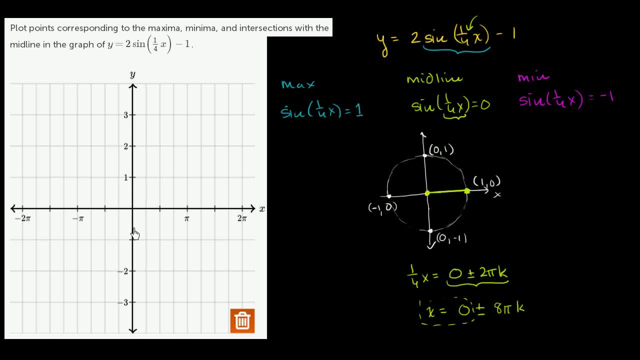 So we have the midline right over here: x equals 0.. y is equal to negative 1.. And we're also hitting the midline right over there. Now let's think about a maximum value. So if we have a maximum value, we're going to have a maximum value. 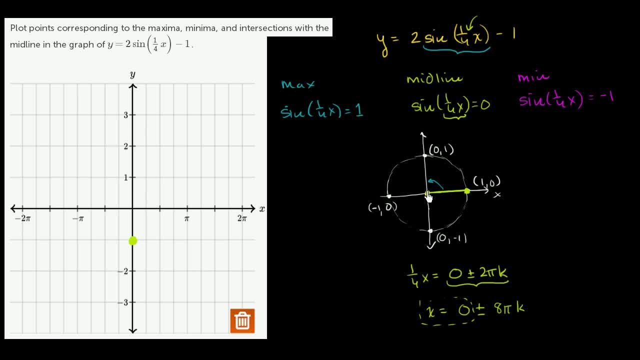 So if we have a maximum value, we're going to have a maximum value. So if we increase our angle right over here all the way to pi over 2 radians, we get to this point right over here. Sine hits its maximum value whenever. 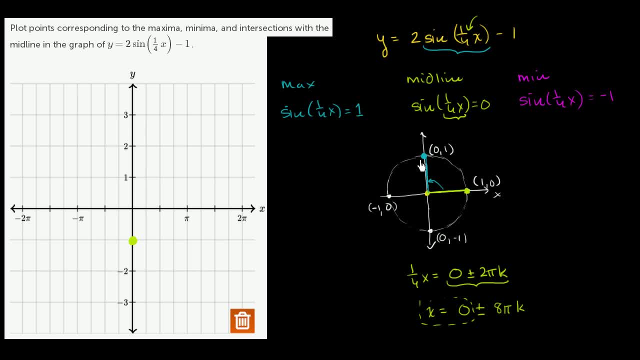 we're taking the sine of pi over 2 plus or minus any integer multiple of 2 pi. So this is going to hit a maximum whenever what we input into the function is equal to pi over 2 plus or minus some integer multiple of 2 pi. 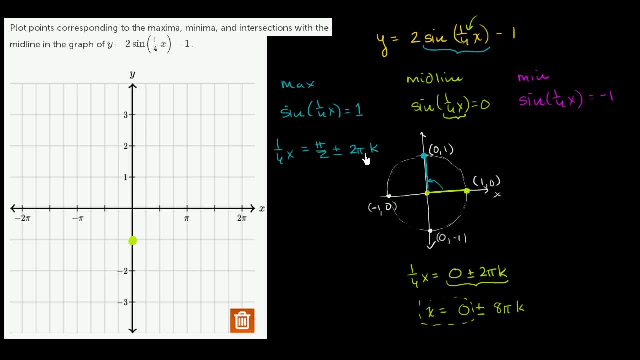 Well, once again, multiply. Multiply this by both sides, by 4.. You get: x is equal to pi over 2 times 4 is 2 pi plus or minus 8 pi k. Now which x value would we want to do? 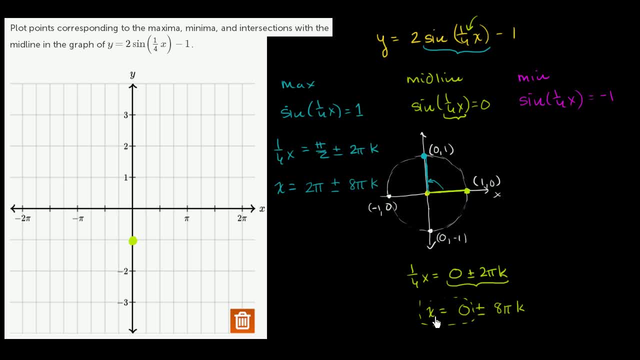 Well, actually even the last one, I picked x equals 0 for simplicity. But if I did, x equals 8 pi or 16 pi, those aren't even on this graph. Or if I want to do, x is equal to negative 8 pi. 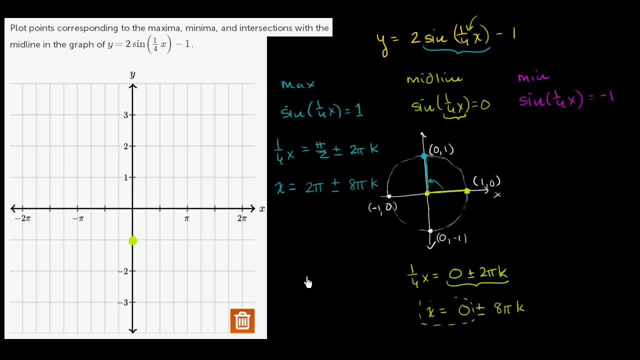 those aren't even on the graph, So this is actually the only one that sits on this graph, Likewise over here. So over here, x equals 2. pi is the only one that's actually on this graph. If I added 8 pi, I would go off the graph. 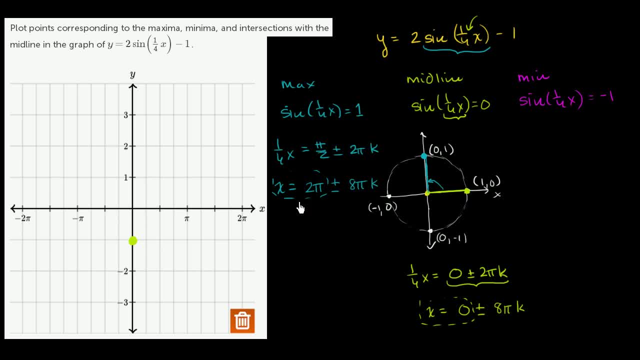 If I did 2 pi minus 8 pi, at negative 6 pi, that's off the graph. So I'm going to do x equals 2 pi When x equals 2 pi, 1 fourth of 2 pi is pi over 2.. 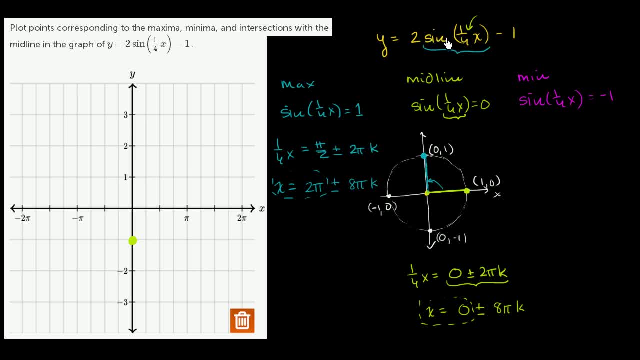 Sine of pi over 2- we've already saw- is 1.. 2 times 1 is 2 minus 1 is 1.. So when x is 2, pi we're at the point y. y is equal to 1.. 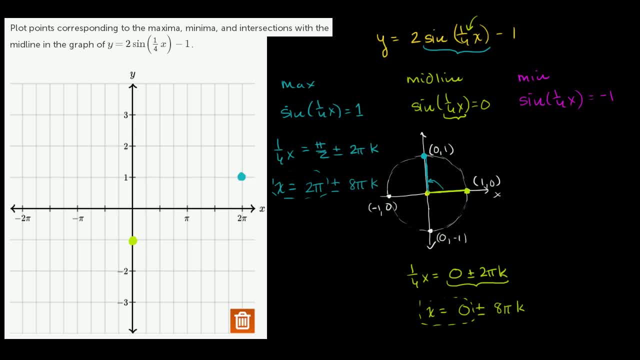 That is a maximum point. And then, finally, same logic for the minimum point. We need to see when this 1, fourth x hits not pi over 2, but now negative pi over 2.. We could have also picked 3 pi over 2 if we wanted. 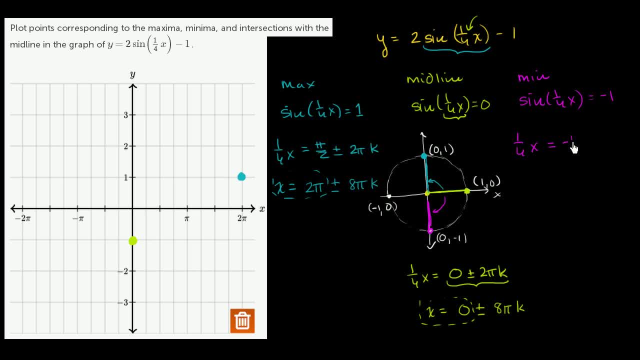 So negative pi over 2 is equal to negative pi over 2, plus or minus any integer multiple of 2 pi. So once again, multiply times 4, x is equal to negative 2 pi, plus or minus 8 pi, some integer multiple of 8 pi. 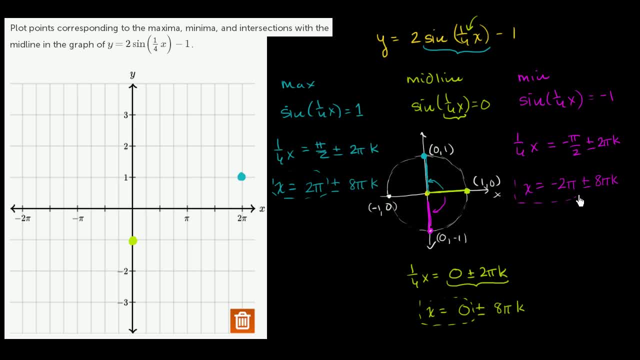 So, once again, the only of these that's actually on our graph is: x is equal to negative 2 pi. When x is equal to negative 2 pi, what does our function equal? Well, 1. fourth, We already know that when x is equal to negative 2 pi, 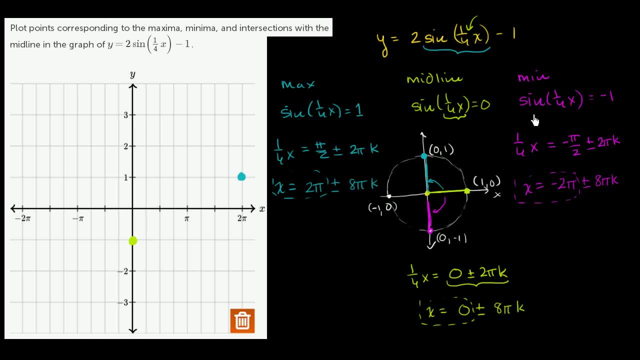 1. fourth x is going to be equal to negative pi over 2, sine of negative pi over 2 is negative 1.. 2 times negative 1 is negative. 2 plus negative 1 gets us to negative 3.. So it's that point right over there. 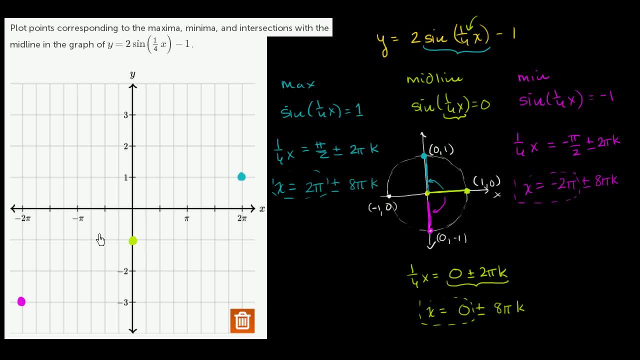 So those are our points, And if we actually wanted to graph, they just ask us to graph these points. But if we wanted to give a little bit more texture here, we could draw the midline right over here at y is equal to negative 1.. 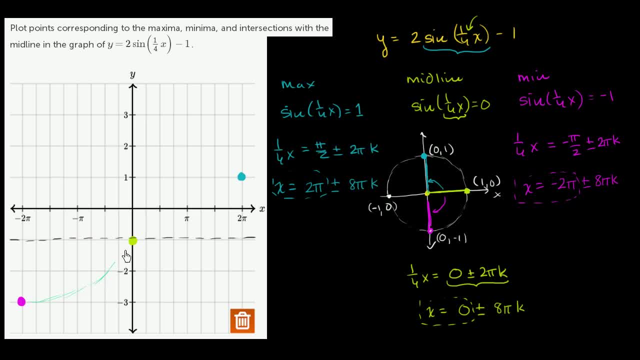 And if we wanted to actually try to plot this function, it would look- or at least the part that we can graph. it would look something like this: But actually, let's just get the tool out And it would keep going if we had more real estate. 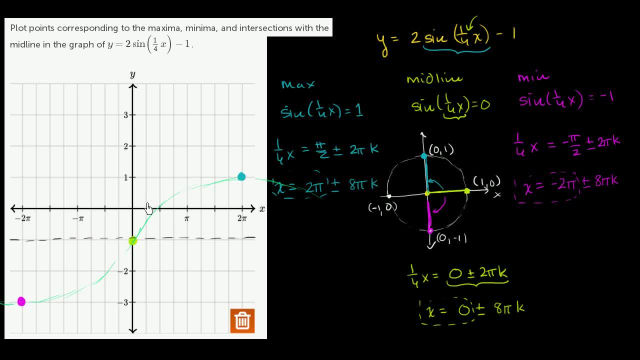 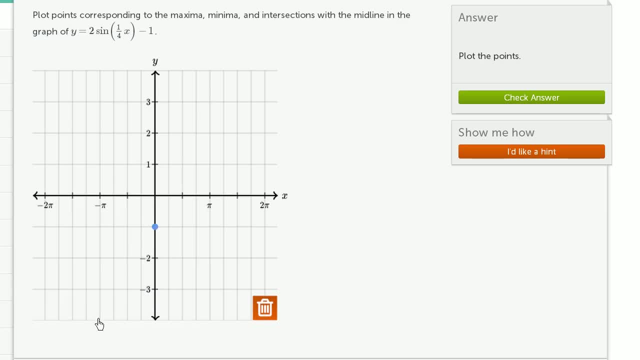 But let's- actually we're not even plotting a complete period here, But let's go back to our tool and plot these points and make sure that we got it right. So we want a point. That's where we intersected the midline. 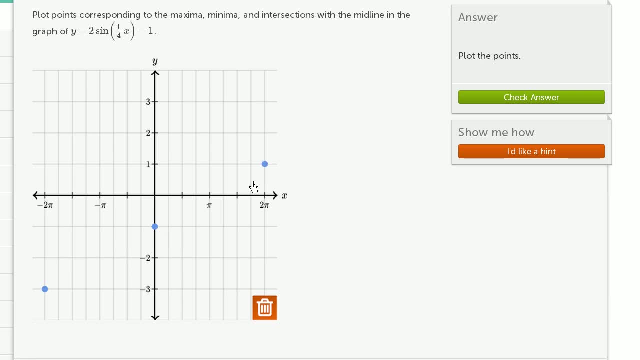 This is our minimum point. That's our maximum point based on what I just did. Check the answer. We got it right. 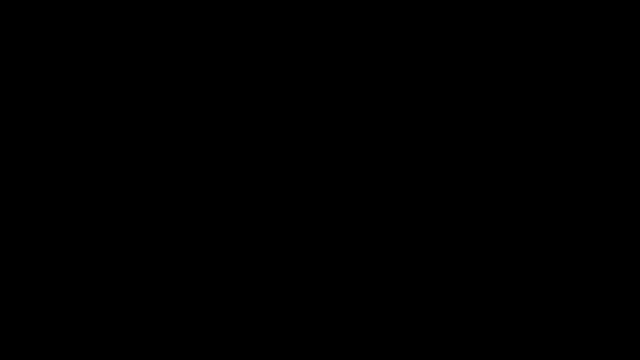 In this video we're going to talk about how to find the surface area and the volume of a square-based pyramid and a triangular pyramid. So let's draw a picture of the square-based pyramid- Just a rough sketch- And let's calculate the volume of this pyramid. first,